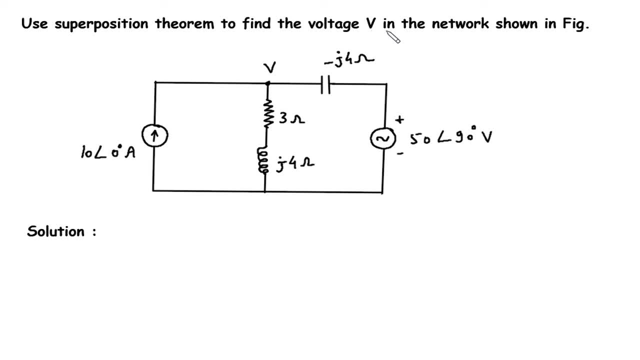 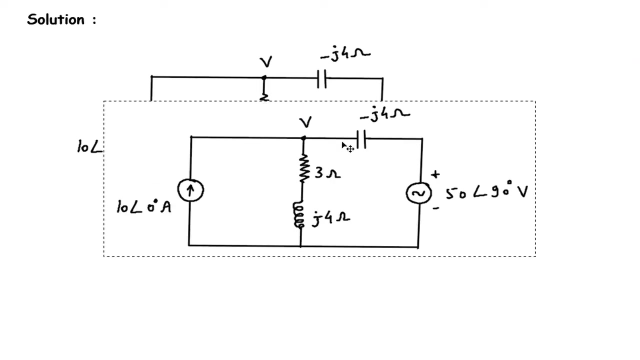 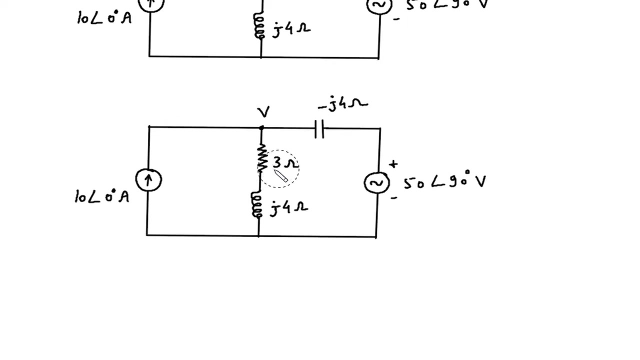 Use superposition theorem to find the voltage V in the network shown in figure. We have to find this voltage using superposition theorem Solution. first of all, we will find impedance of this branch and impedance of this branch. So this will be, let's say this is Z1 and 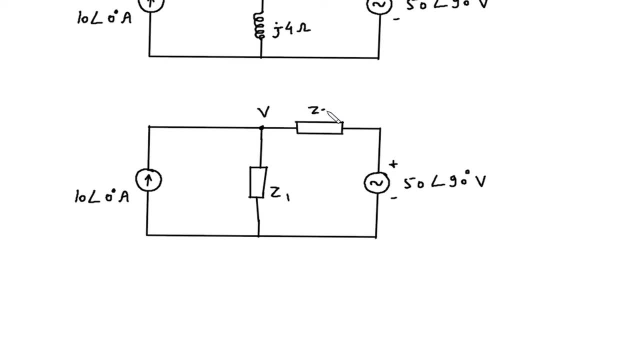 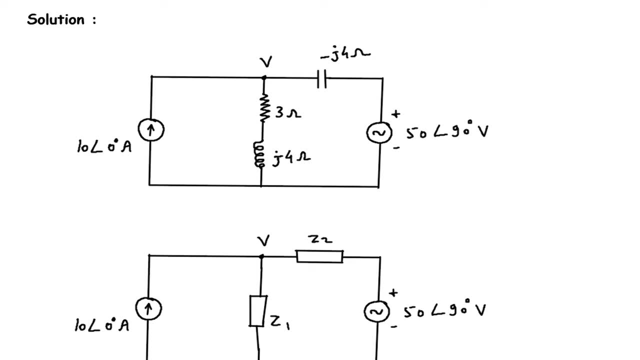 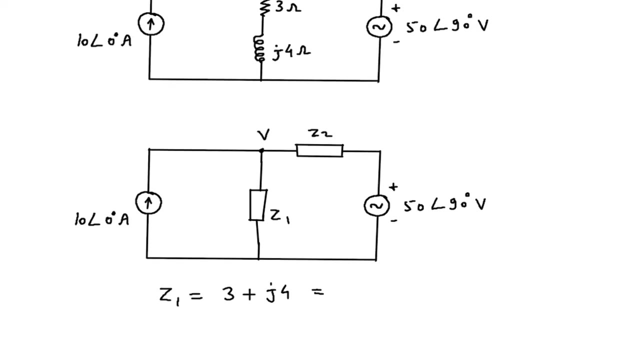 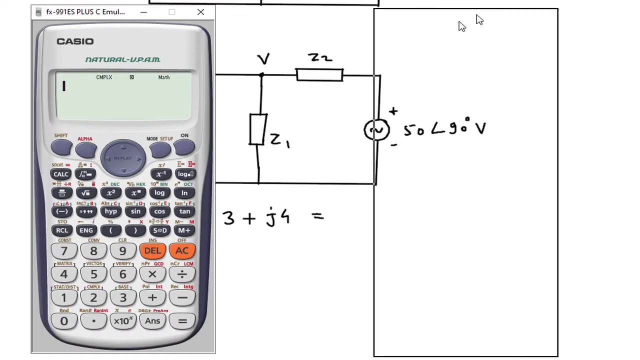 this is Z2.. Now Z1 is equal to 3 plus J4.. 3 plus J4. It is in rectangular form. We can convert this into polar form. So in polar form this will be mode, then complex mode. So 3 plus. 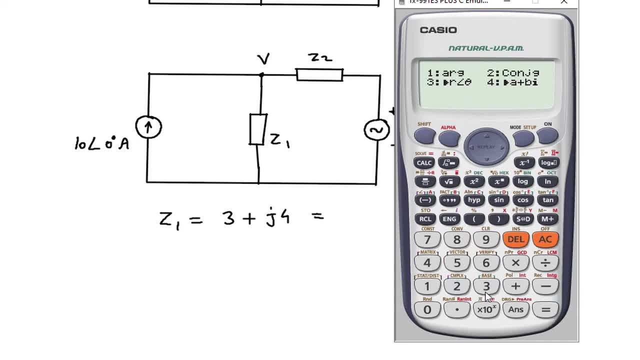 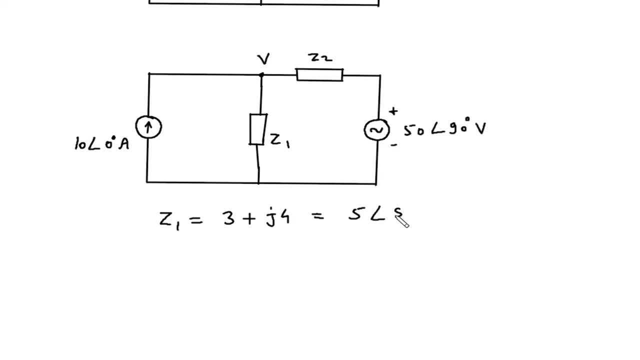 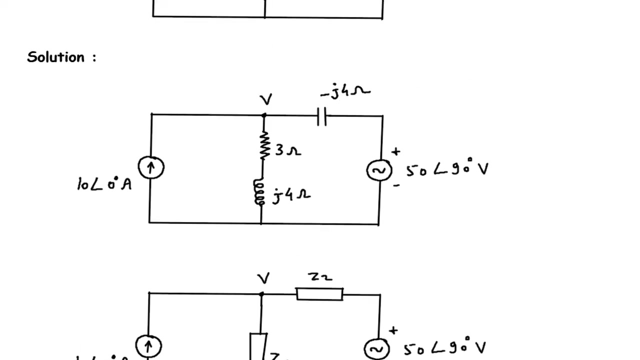 I into 4.. Shift 2, then 3.. So it is 5 at an angle of 53.. 5 at an angle of 53.13 degree. This is the value for Z1.. Then Z2 is minus J4.. Z2 is minus J4.. 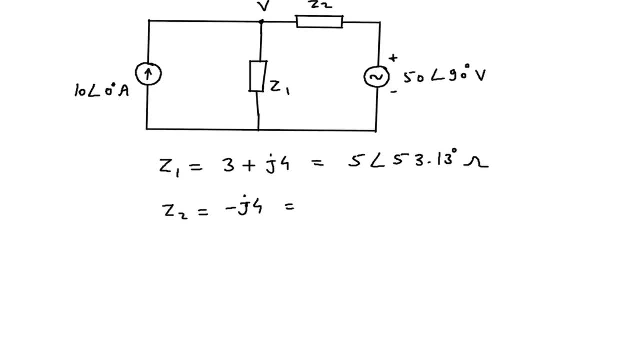 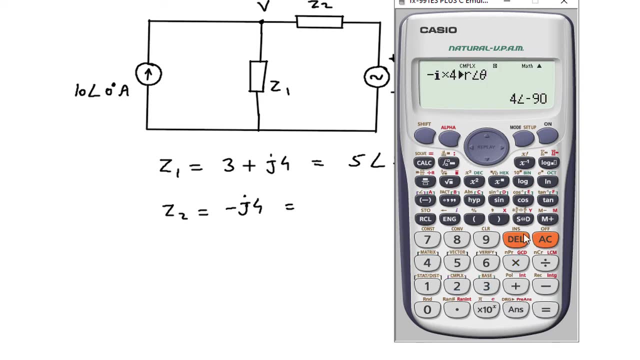 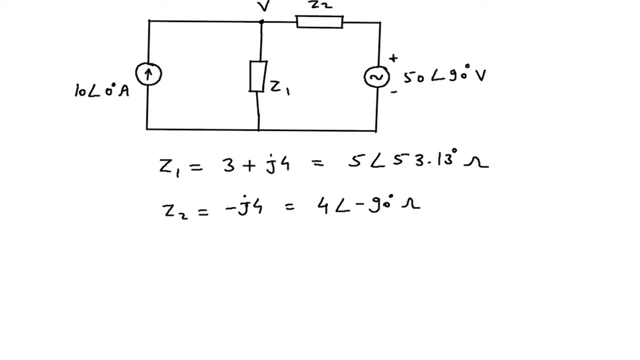 So minus I into 4.. Shift 2, 3. It is 4 at an angle of minus 90 degree. This is the value for Z2.. Now we have to use superposition theorem here, And this is an AC circuit because it 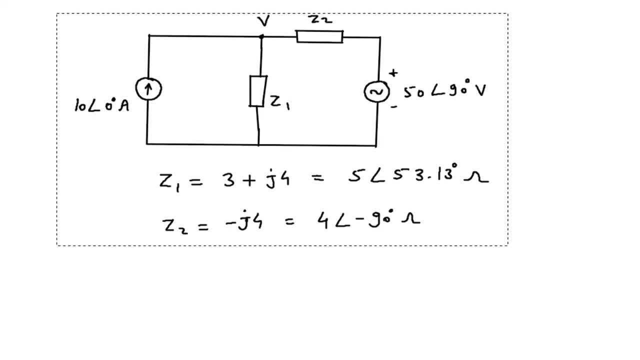 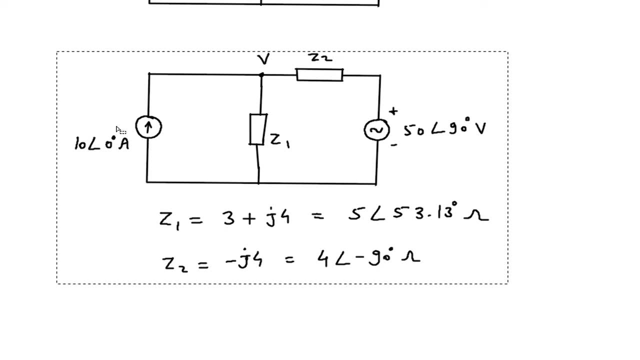 contains an AC source. Now we will consider first, let's say we will consider this current source first. So consider this 10 ampere, 10 at an angle of 0 degree ampere- current source and turn off all other sources. Now we'll look at this. 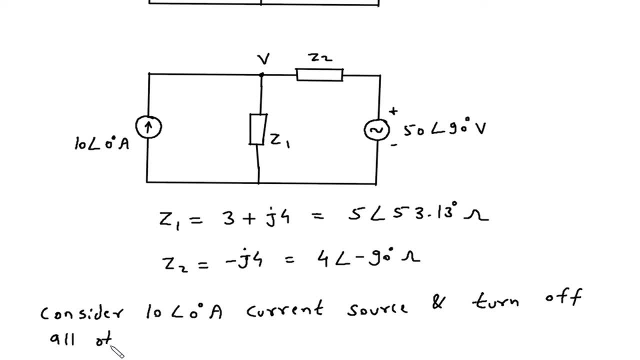 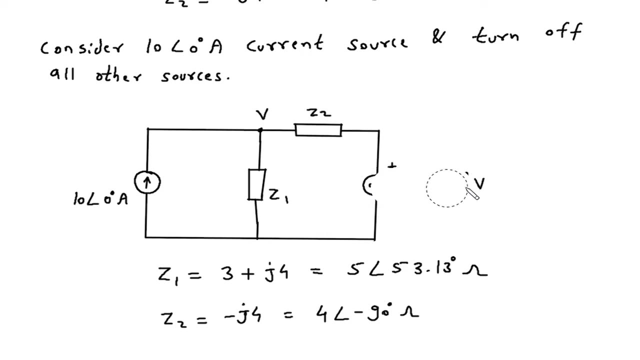 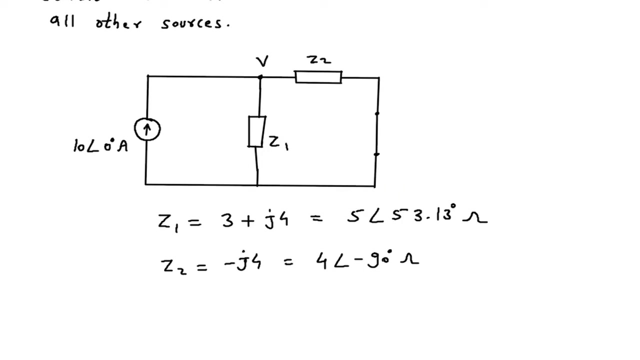 I will use this as the current source, All other sources. Now, if we turn off this voltage source, this will be short circuited, So we can replace this with a short circuit. Now, here we can see this: Z1 and Z2 are in parallel. 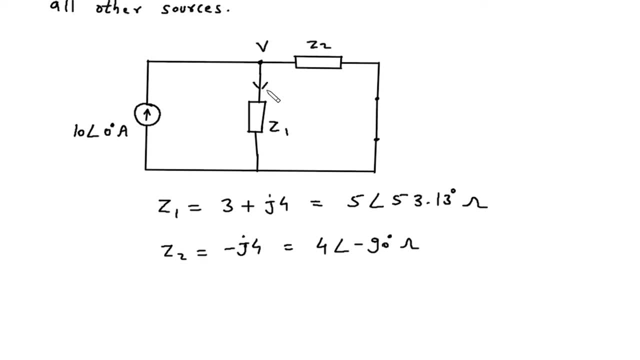 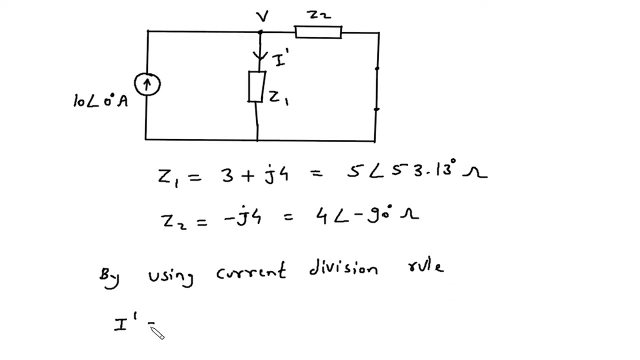 Or we can use current division rule here. Let's say this is current I', So we can find I' using current division rule by using current division rule. So I' is equal to this current, that is, 10 at an angle of 0 degree. 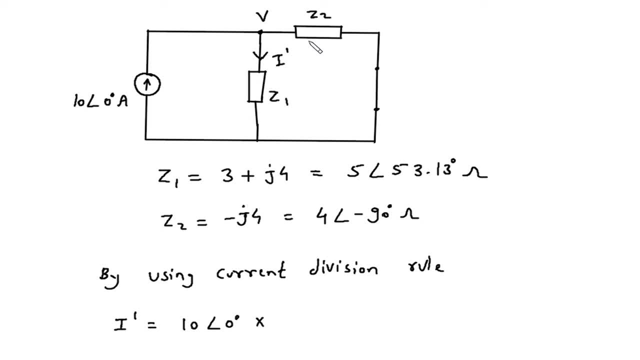 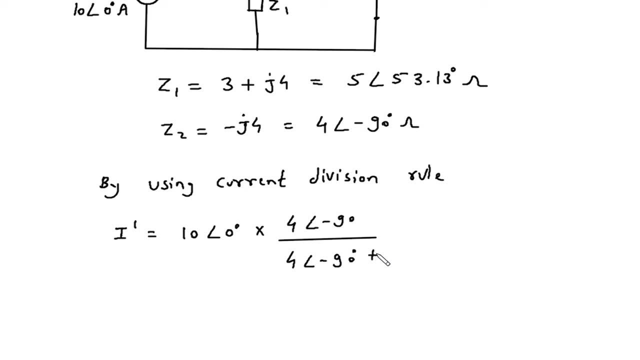 So I can write I' into opposite branch resistance, that is Z2.. And Z2 is 4 at an angle of minus 90 degree divided by same 4 at an angle of minus 90 degree, Then plus. Here we can see we can use here rectangular form of this Z2, that is minus J4.. 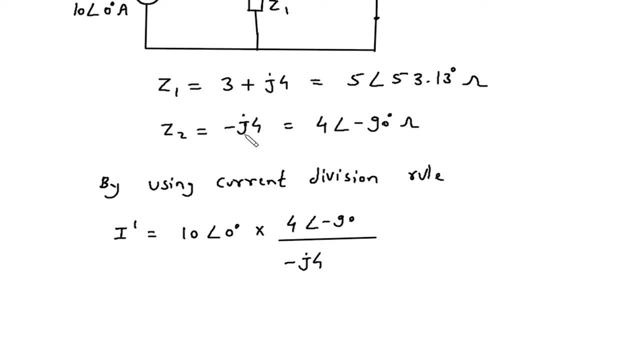 Because addition and subtraction are better perform in rectangular form and multiplication and division are better performed in polar form. so here in denominator we have to use addition, so we will use rectangular form here. so minus j4, then plus z2 plus z1, and z1 is again in rectangular form. z1 is 3 plus j4. 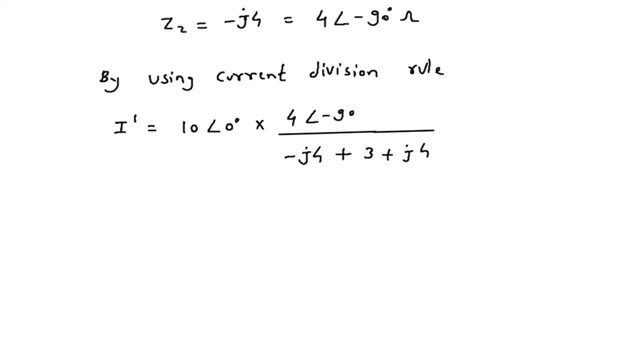 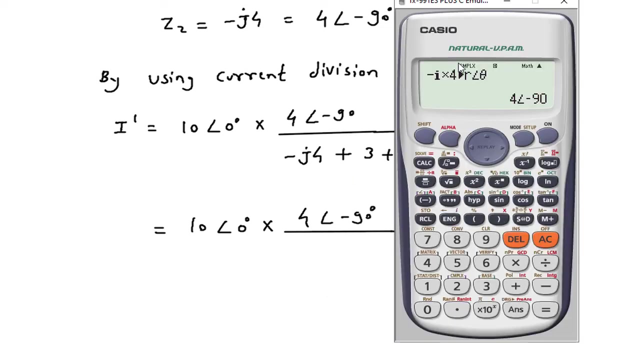 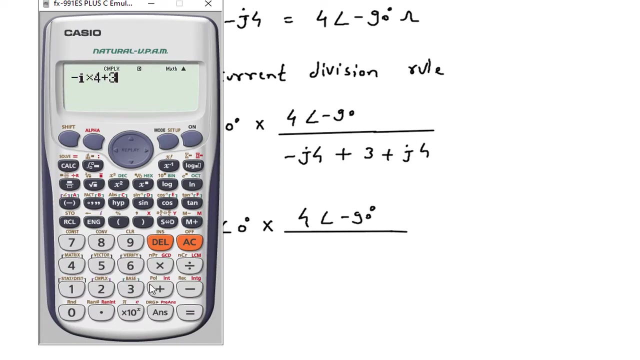 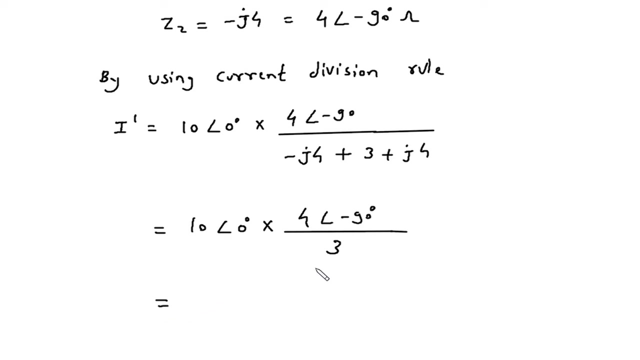 so this will be 10 at an angle of 0 degree into 4 at an angle of minus 90 degree. divided by this will be minus i into 4, then plus 3, then plus i into 4, i into 4, plus 3 plus i into 4, so it is 3. now we can directly substitute this value in calculator. 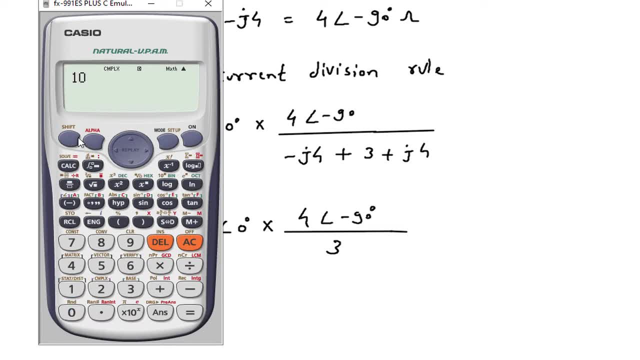 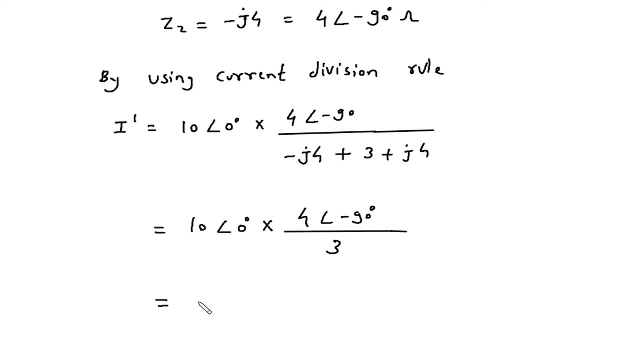 so 10 at an angle of 0 degree. this is in one bracket. then multiplied by in bracket 4 at an angle of minus 90 degree, divided by 3, so it is minus 13.33, minus 13.33 j. this is the value for i prime. it is in rectangular form. in polar form, this will be: 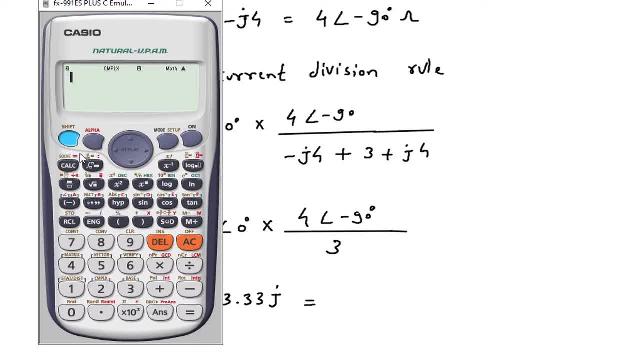 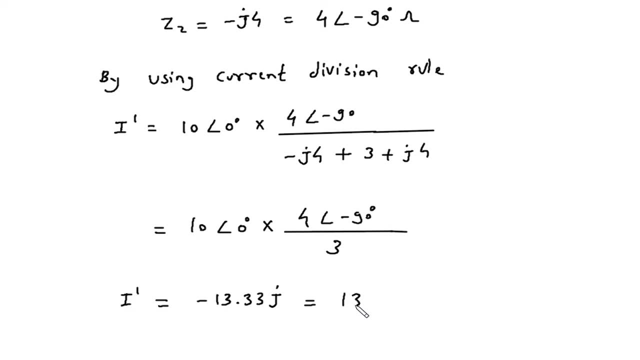 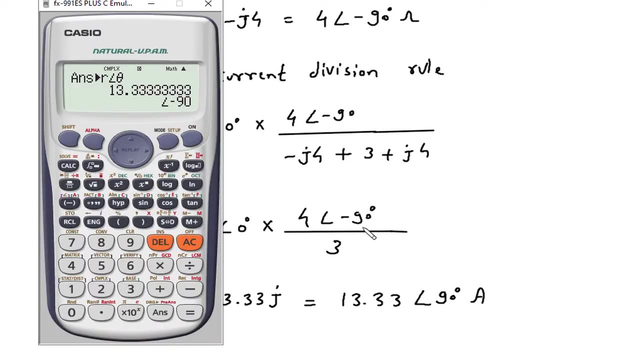 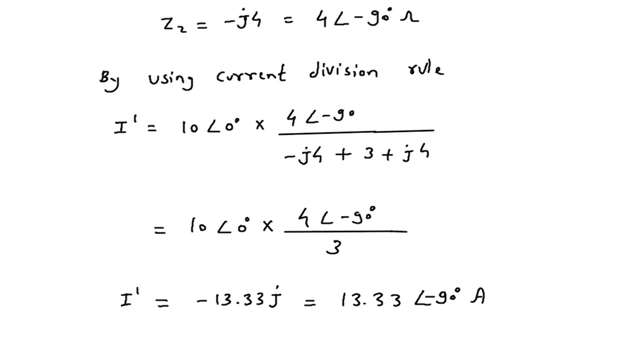 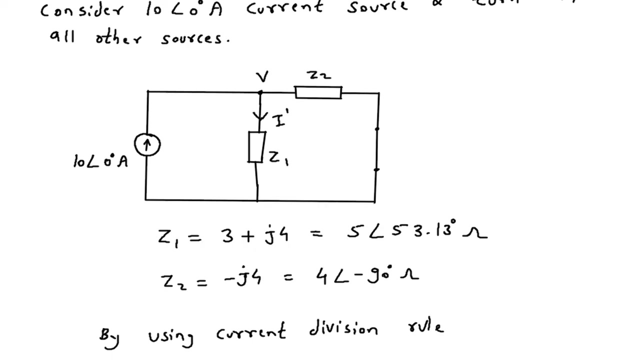 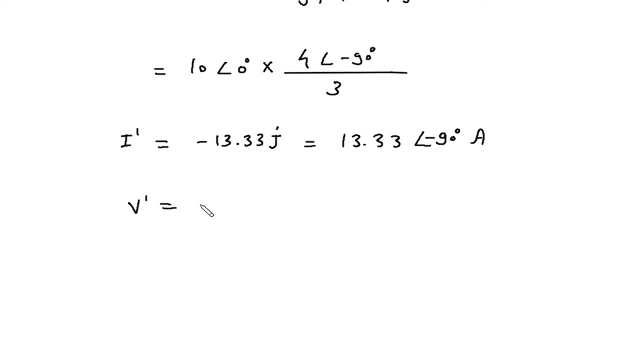 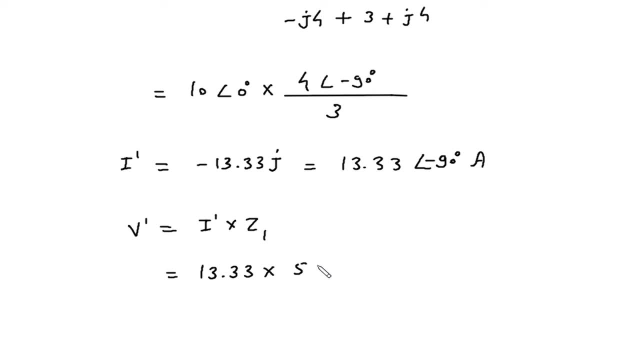 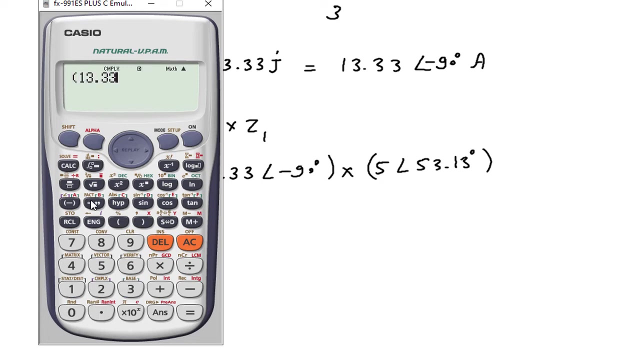 5 at an angle of this is 13.33 at an angle of minus 90 degree. then into z1 is 5 at an angle of 53.13 degree. so this will be in one bracket: 13.33 at an angle of minus 90, multiplied by 5 at an angle of 53.13, bracket complete. 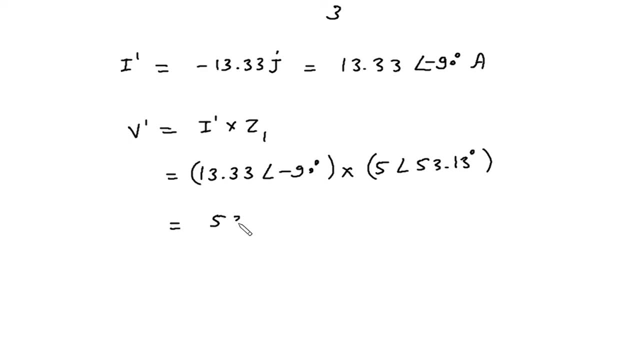 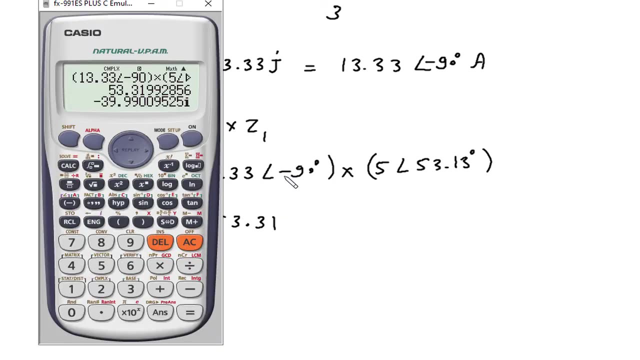 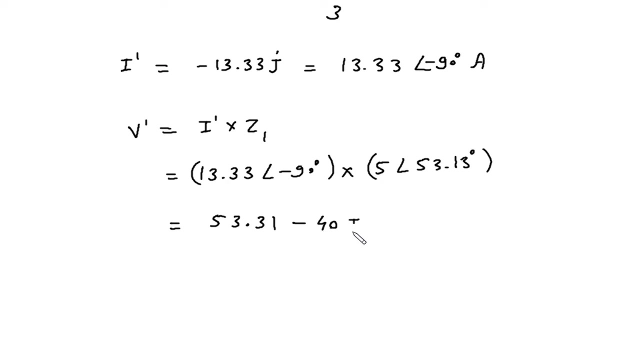 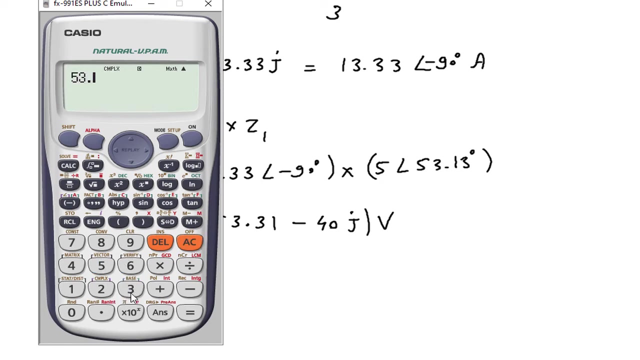 So it is 53.31. then minus this, minus 39.99, we can write 40. so minus 40 j. This is the value for v prime in rectangular form. Then in polar form this will be 53.31.. 53.31 plus 40 into i, not plus, it is minus. 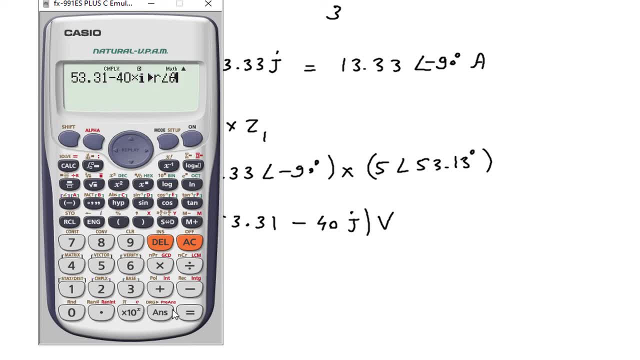 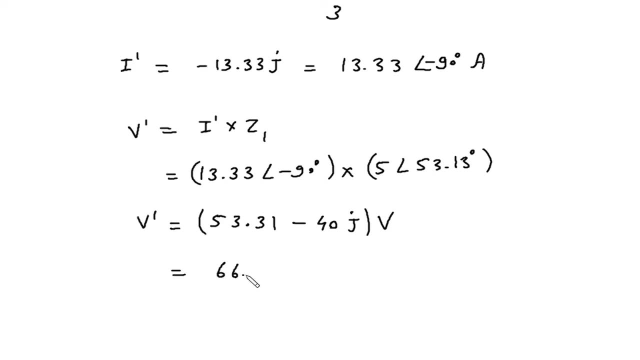 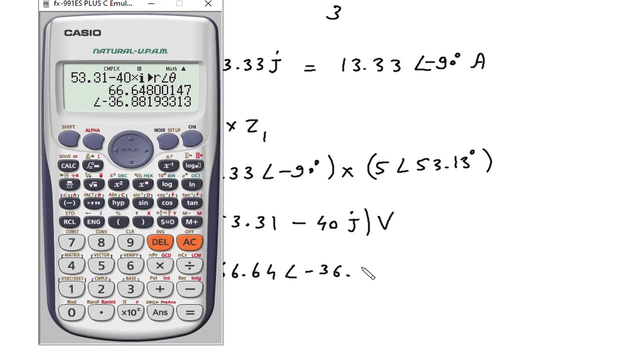 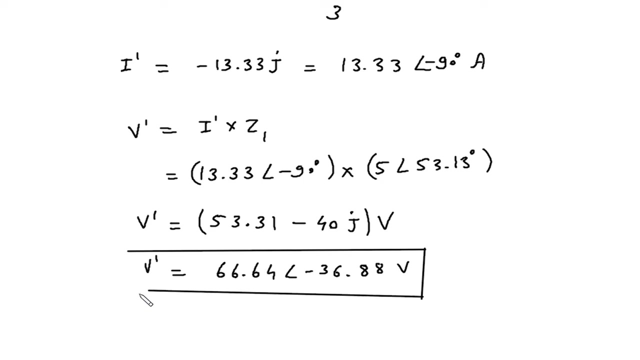 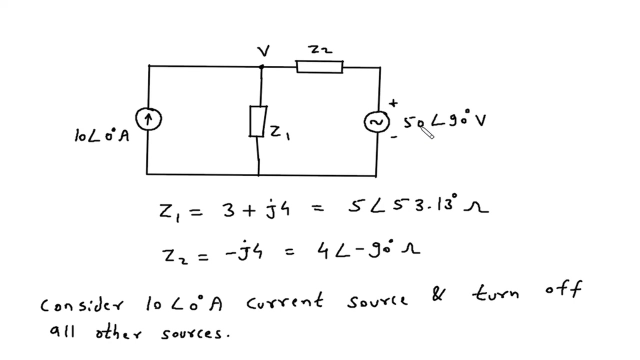 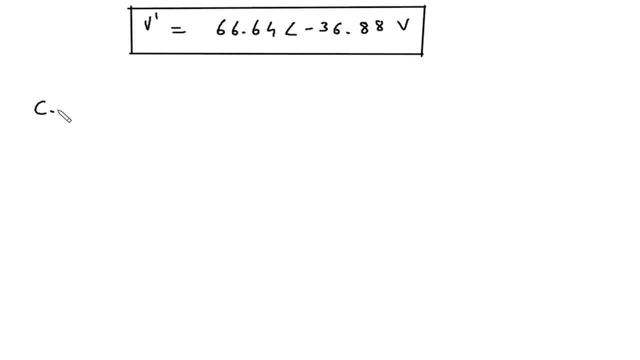 Then shift to 3. So it is 66.64 at an angle of minus 36.88 volts. This is the value of v prime. Then next we have to consider. Next we have to consider This voltage source 50 at an angle of 90 degree volt and turn off this current source to consider. 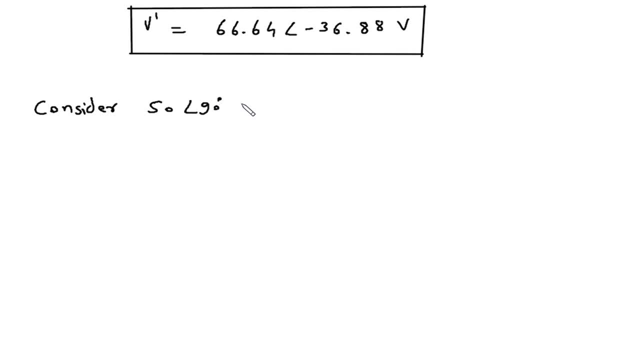 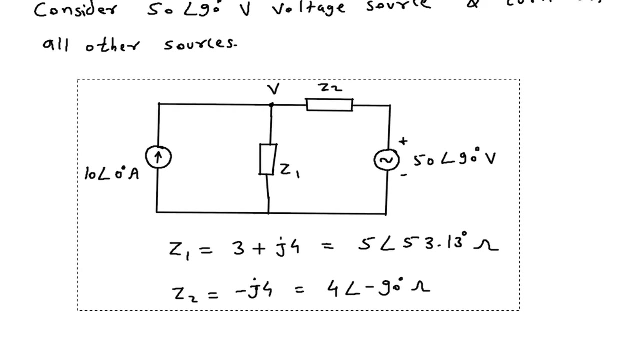 50 at an angle of 90 degree voltage source and turn off all other sources. Now, if we turn off this current source, So this will be open circuit. Let's say this is i double prime and let's say according to the polarity of this voltage: 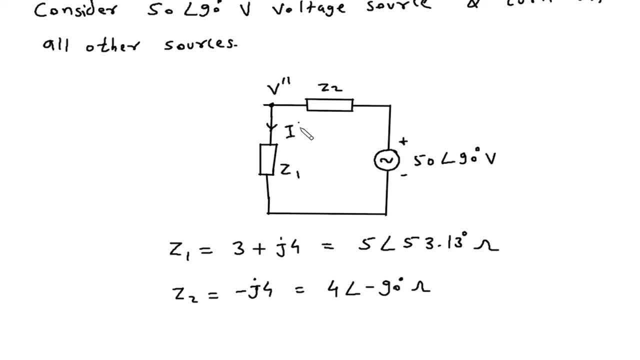 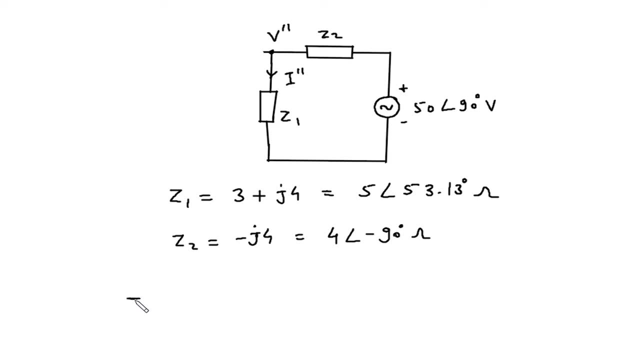 source. Let's say this is the direction of current. Let's say this is i double prime. Now we can easily find this: i double prime by using Ohm's law. So i double prime is equal to v by v by z. So v here is 50 at an angle of 90 degree volt. 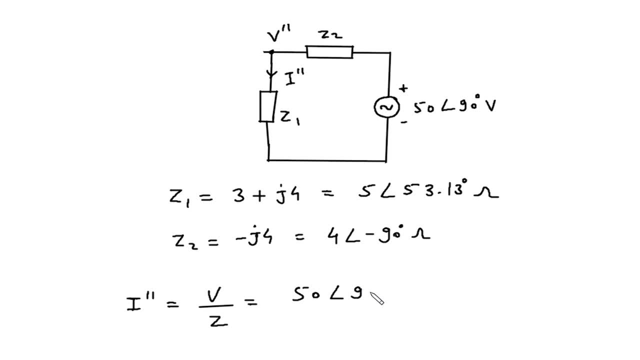 So v here is 50 at an angle of 90 degree volt. So v here is 50 at an angle of 90 degree volt. So it's i double prime And this v here is i double prime flocked to 90 degree. 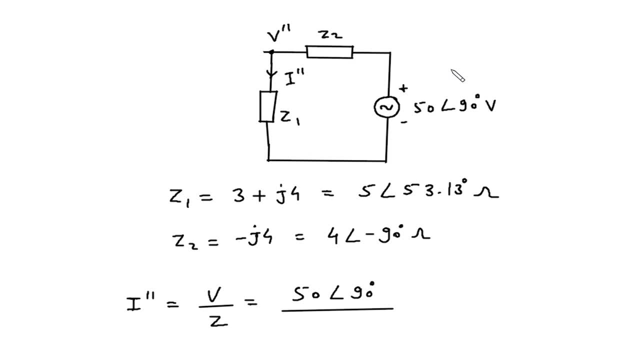 And this v, here is i double prime. And this v, here is i double prime. flocked to 90 degree, divided by z, now z is z1 plus z. Now z1 plus z2 will be 3 plus 3 plus j4, then plus. 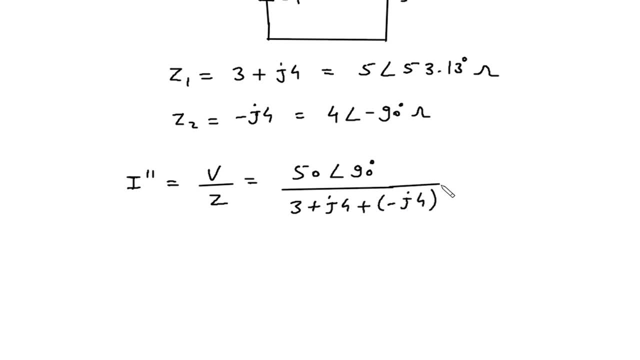 This will be j4. So this will be cancelled. So what's the main? 50 at an angle of 90 degree divided by 3.. So these values over k will very often, And plus j3 over k, will be V2 over the? u talk to make an angle of 90 degree divided by 3.. 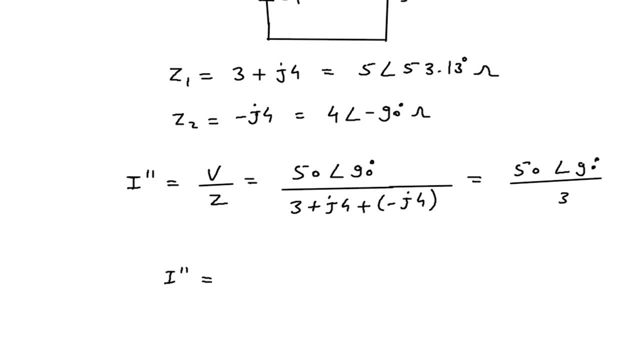 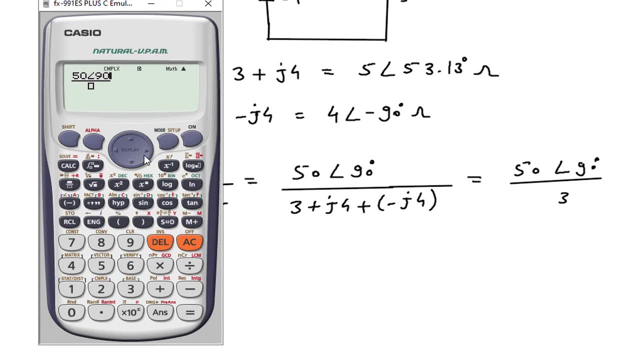 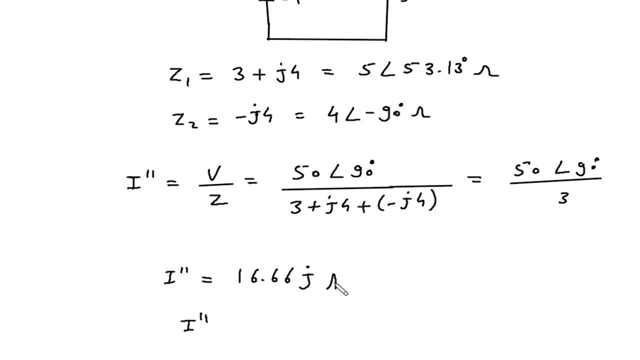 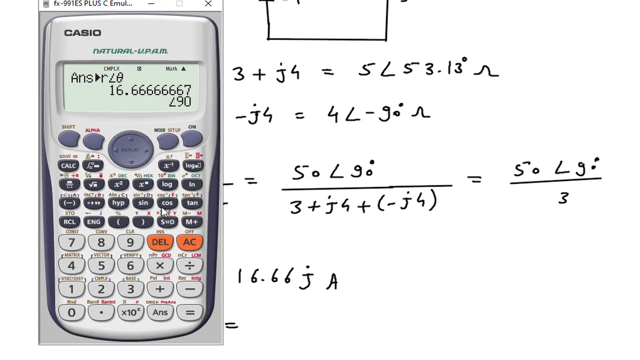 This is the value of I double prime, double prime, I double prime is equal to 50 at an angle of 90 degree divided by 3.. So it is 16.66 j. Now ampere in polar form. this will be shift to 3.. So it is 16.66 at an angle. 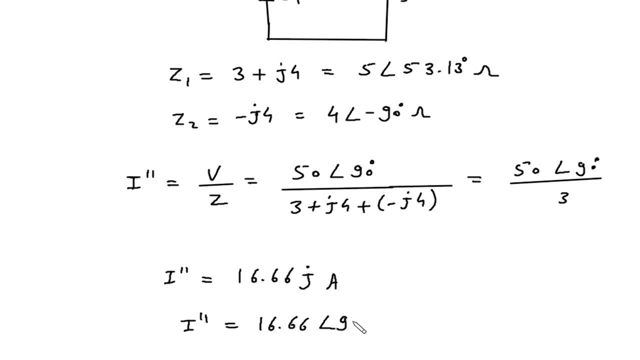 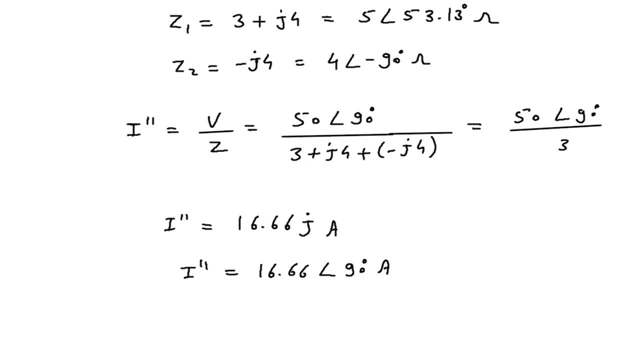 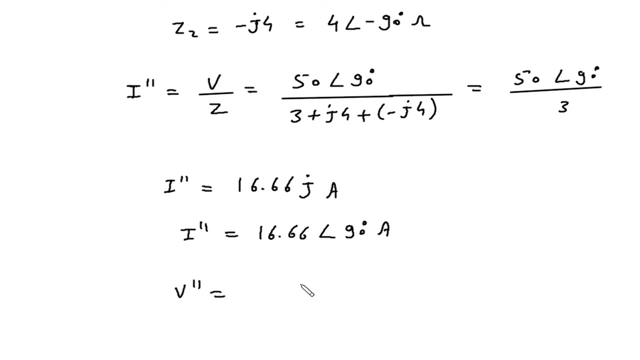 of 90 degree ampere. This is the value of I double prime. I double prime is equal to double prime, But we have to find this V double prime. v double prime will be equal to high double prime into z1. I double prime into z1, so I double prime is again 16.66 at an angle. 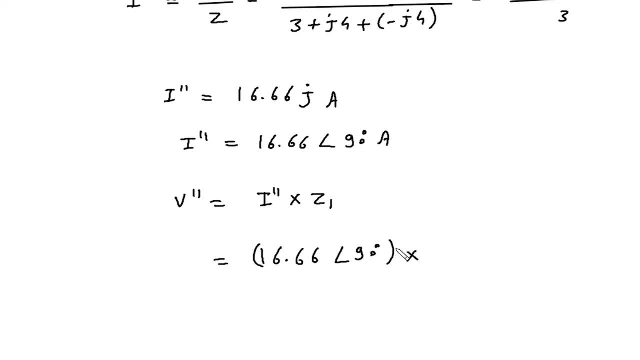 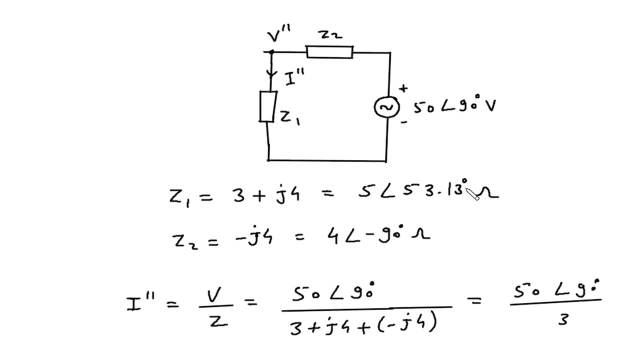 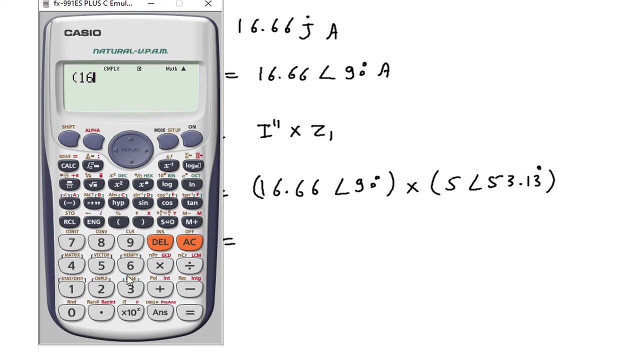 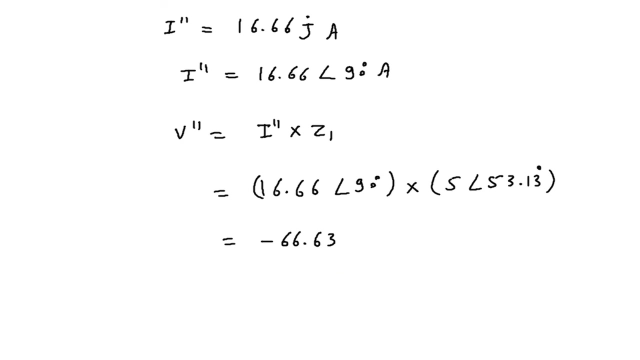 of 90 degree multiplied by Now, z1 is 5 at an angle of 53.13 degree, so this will be in one bracket: 16.66 at an angle of 90 degree, multiplied by 5 at an angle of 53.13, so it is minus 66.63, minus 66.63 plus. 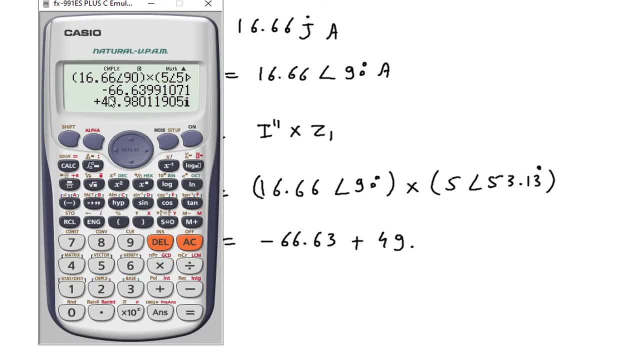 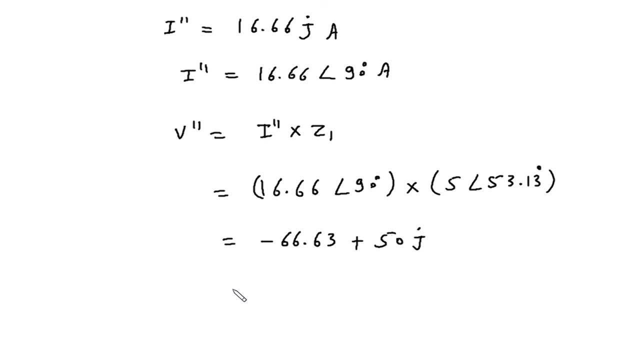 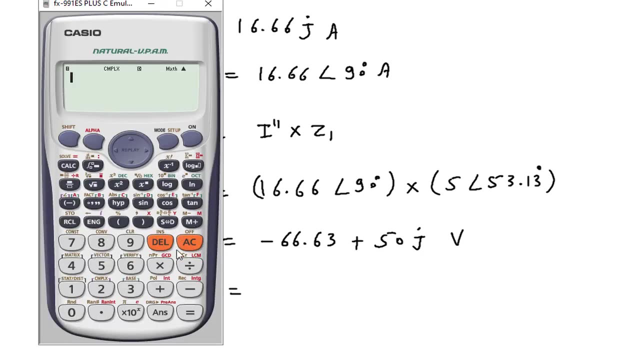 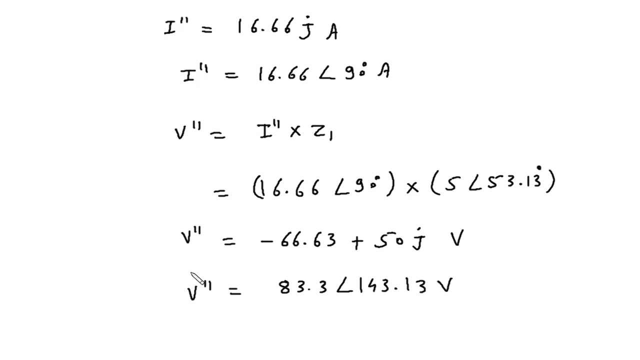 49 point. we can replace this 49.98 by 50 directly, so 50 j. Now this is volt. i double prime now in polar form. this will be shift end, sir, then shift two, three. so it is 83.83 point three at an angle of 143.13 volt. so 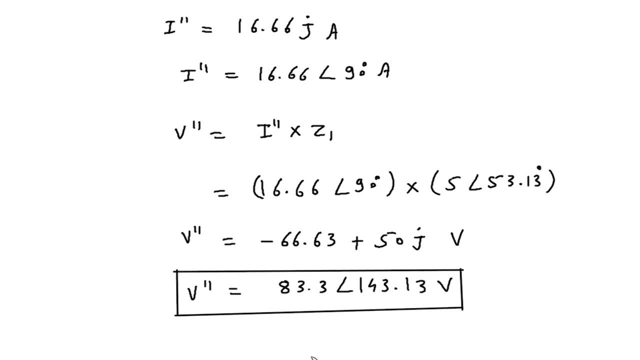 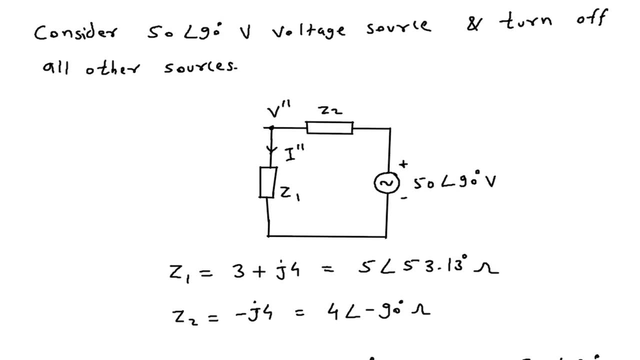 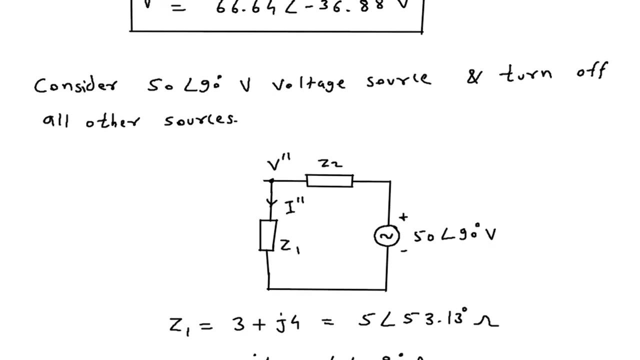 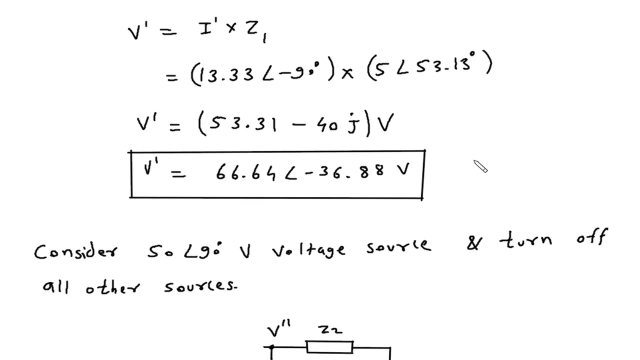 this will be cWhat. this will be cWhat. this is in the dinah bend. so this is cWhat. the is the value of V double prime. Now, here we can see: the direction for I double prime is downward and the direction for I prime is also downward. So we have to add both the voltages. 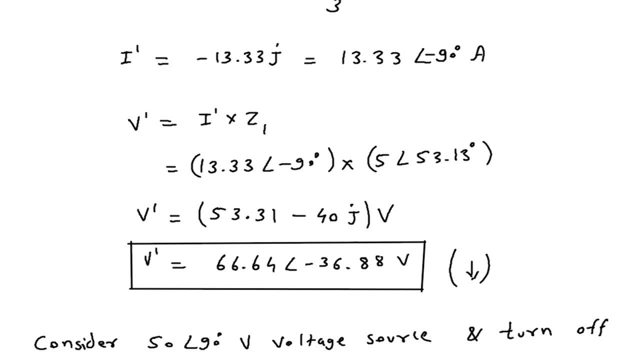 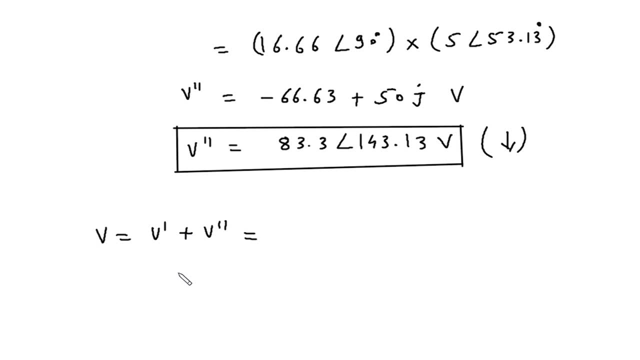 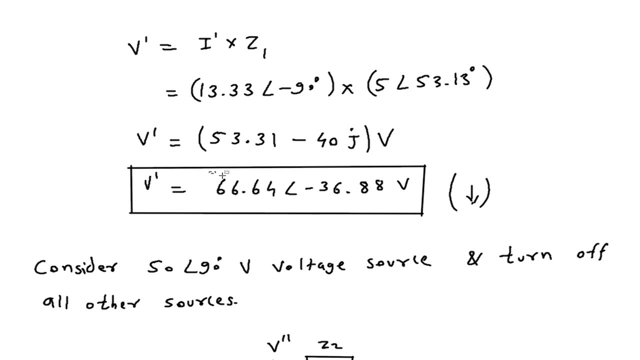 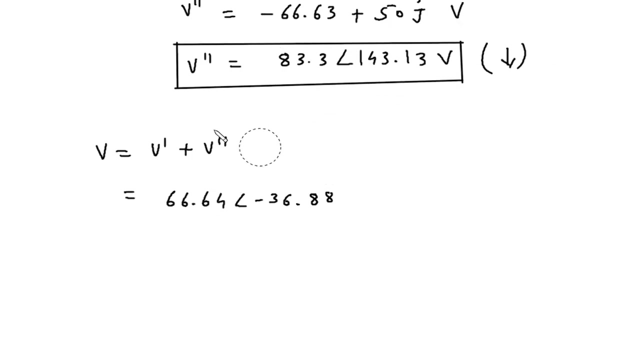 to get the value of this V. So V is equal to V prime plus V double prime. Now V prime is: this is the value for V prime then plus V double prime. So here also we can see that we are doing here addition, So addition and. 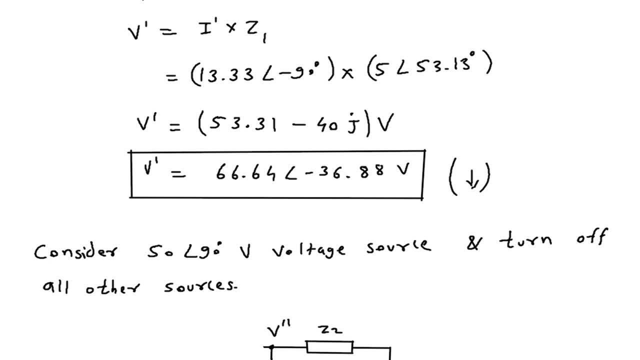 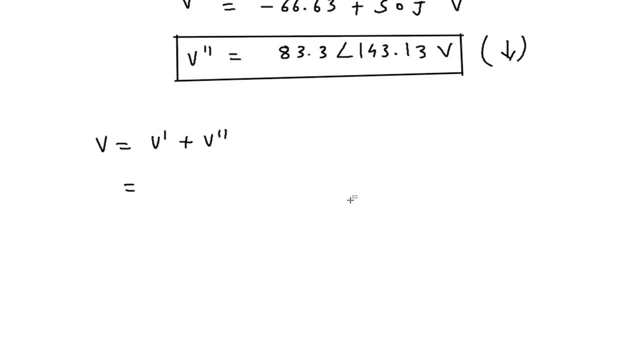 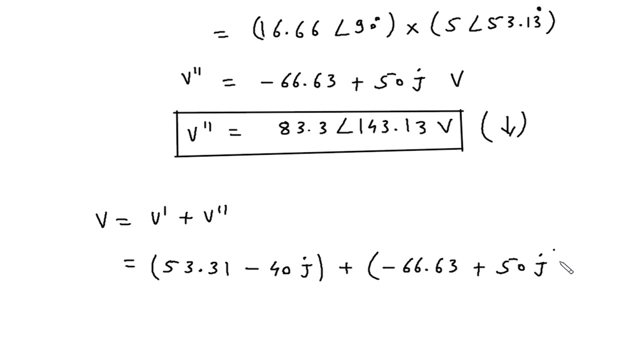 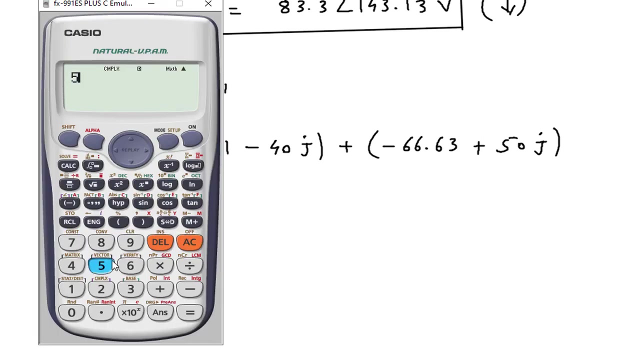 subtraction are better perform in rectangular form. So we will take this value, this rectangular form value, for addition of this V prime and V double prime, then plus V double prime. This is adding both this I double prime and minus I double prime, and that helps me to get this. So I have to pass B by V double prime, b by I double prime. 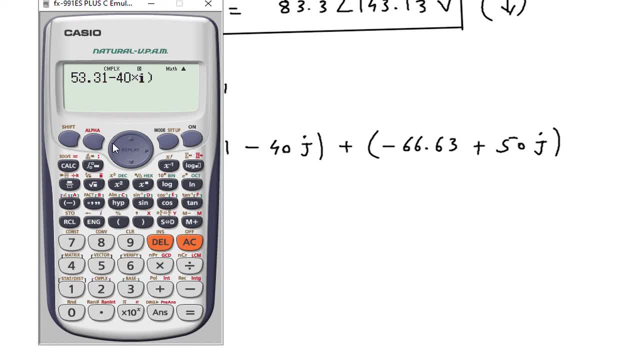 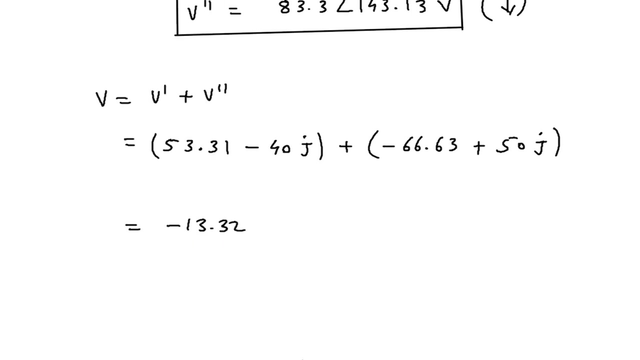 So how I am going to do in this type congress. Let me just sort Then plus in bracket minus 66.63 plus 50 into i bracket complete. So it is minus 13.32 minus 13.32 plus 10j. this is the value for v.